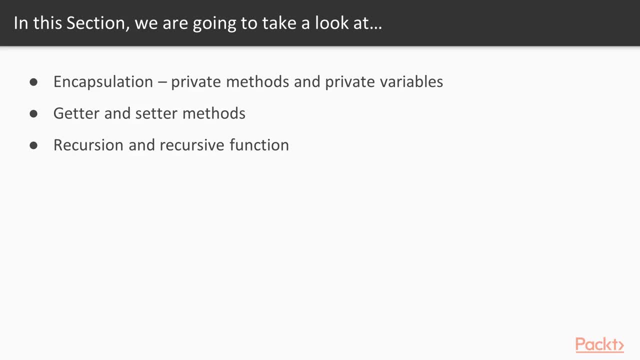 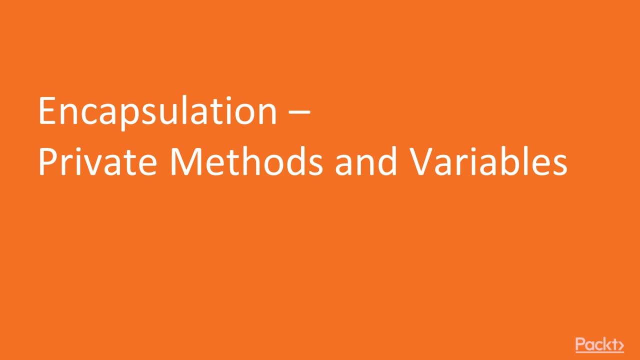 to encapsulation and its benefits, followed by learning the principle of private methods and private variables, then moving on to essentials of getters and setters method and finally familiarize you with the concept of recursion. With this overview, we will lead into the first lesson that deals with encapsulation and private methods and variables. I am pretty 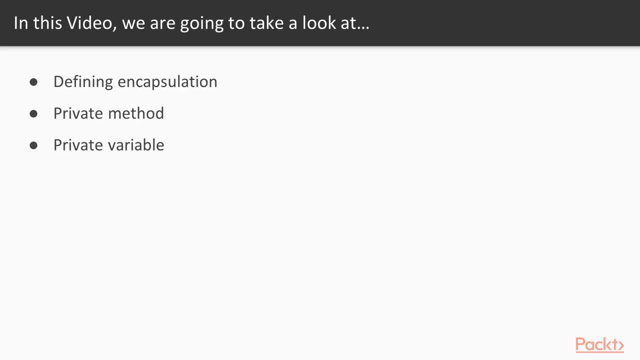 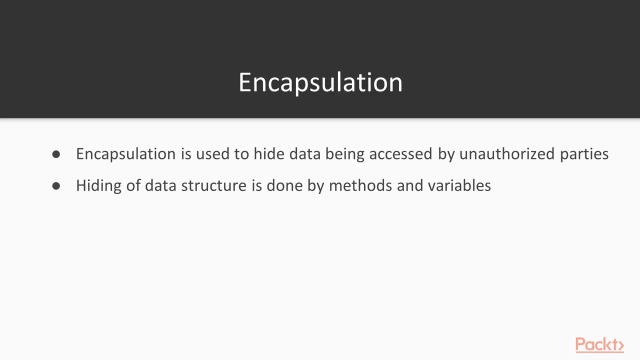 sure all of us has been in the following situation before To write a complex piece of program. in this video we are going to learn first defining encapsulation in Python, Then we will move on to private method understanding and last with private variables. I am pretty sure all of us has been in the following situation before You write a complex 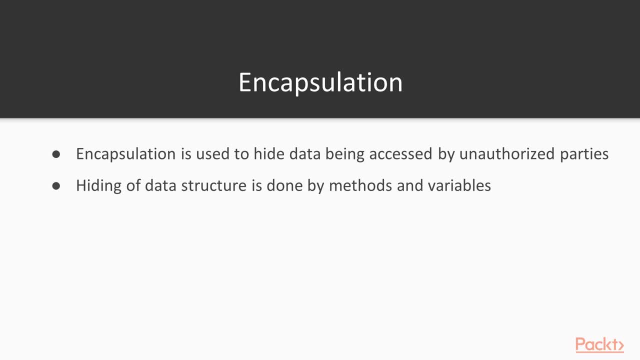 piece of code, but some data gets accidentally modified and you are left with bugs you don't know the location of. To avoid such dilemma, object oriented programming allows coders to restrict access to certain methods and variables through technique of encapsulation. So right now we will get started our first lesson in an example. 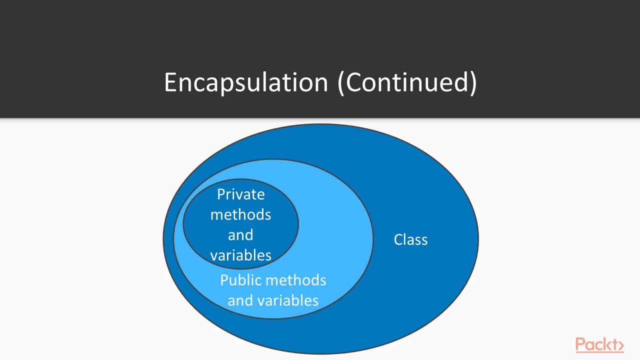 I am just going to describe the concept of encapsulation with different methods and variables. You can see that it is not a simple expression, but a beautiful statement. Finally, I am going to explain the concept of encapsulation of a particular variable and its costs. 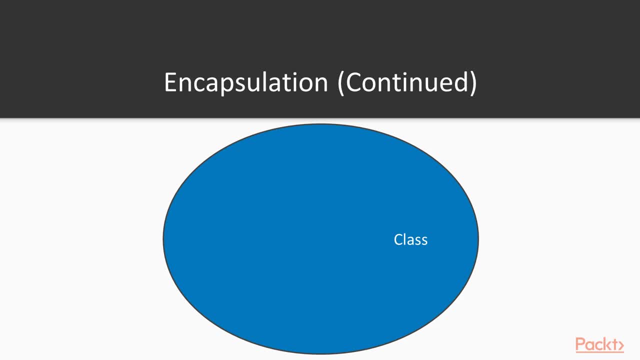 Beispiel 1 by two: An sunny day, a man outside the home. He looks around a faraway place and sees something. I see a giant beech tree. I see a tree, I see a few trees. I see a mountain. 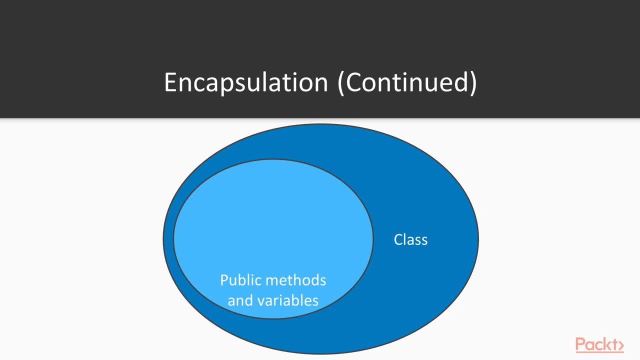 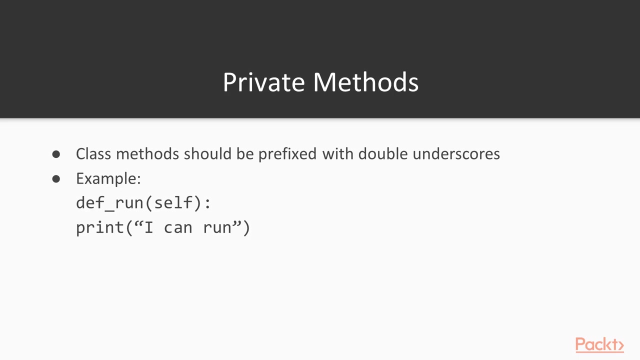 I see a chicken under a syntax utilizing double underscore which will look with an simple program. you will understand those syntax. variables or methods come under private methods and variables which comes under public methods and variables. you will understand this diagram as we go through a simple program code. class method should be prefixed with double underscore. example that: 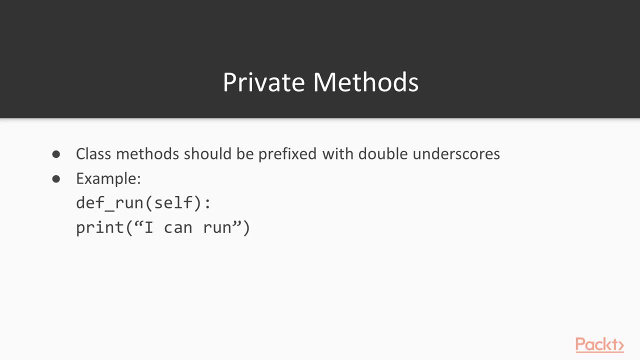 I can give you right now is when we define a run method, we need to define that run method using double underscore with a self-declaration, and then we can use any kind of pass or a print command under it. for a better understanding of private methods, we'll take a simple program. 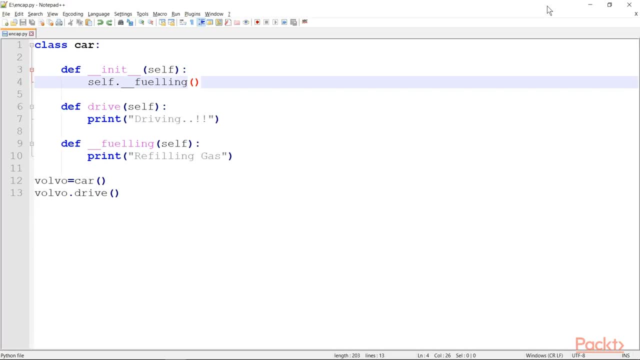 consider the following piece of code that I have already written on notepad plus plus. as you can see, one of the methods in class car is defined with a different syntax. this is how you define a private method. remember a private method is always have the name of the method prefix with double underscore. also, you need to define class variable method. 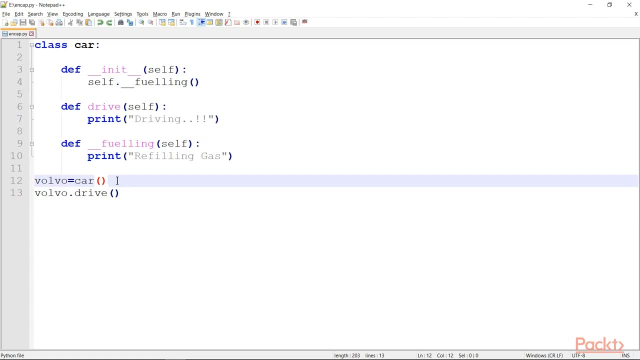 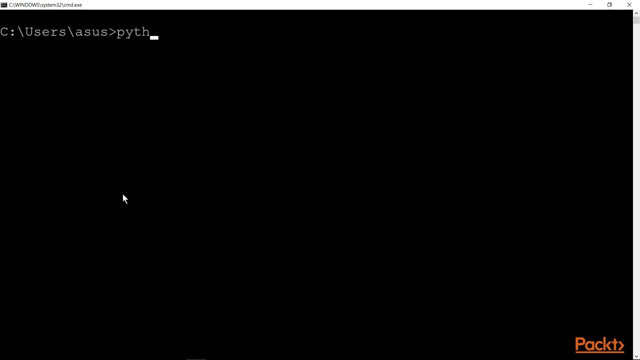 under object declaration. so whenever we declare an object- for example Volvo is declared to the class car- then we can call through an object attribute, that is drive. let's run the program and understand the execution of this program, which will give you an exact print output on our screen. we'll run this program by mentioning the file name that I have given as ncap. 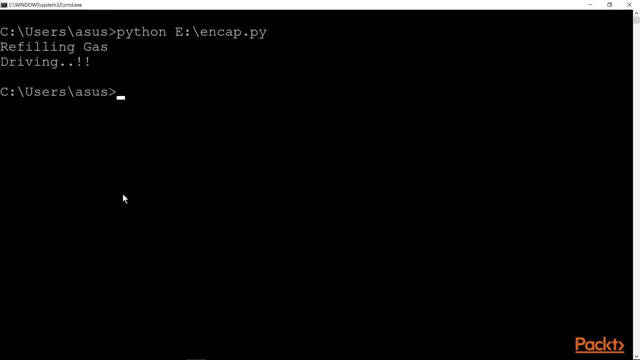 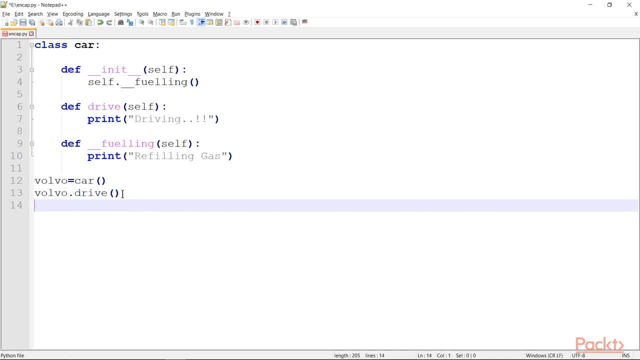 now you can see we have an output saying refilling gas, which is getting utilized by init function, and second output is driving that we have declared in dev drive. let's make a quick change into the same program. we'll mention the object, Volvo, under which we'll try to call the fueling method, for that we have. 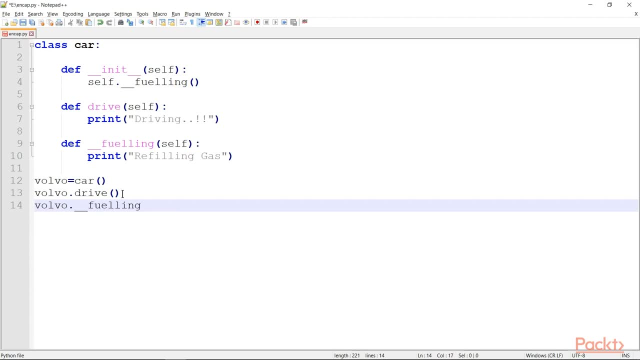 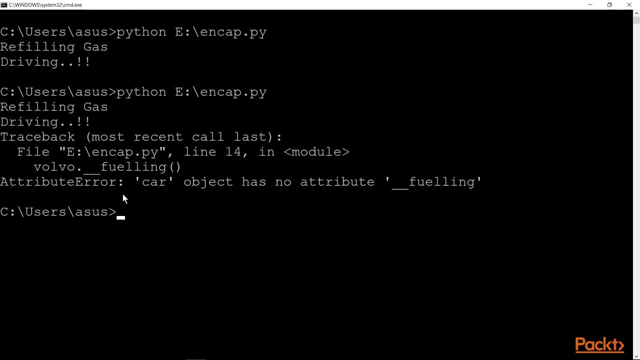 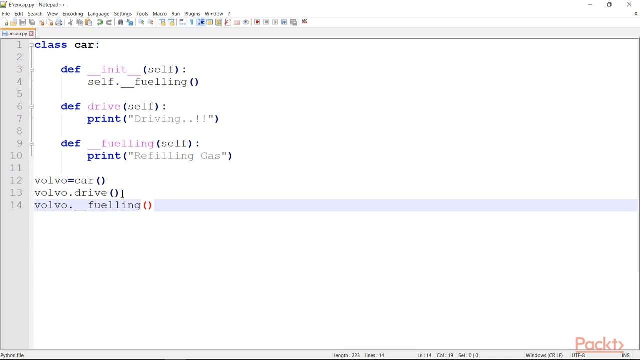 to give double underscore fueling as a syntax. we'll try to save this program and rerun this program using the same code. now that you can see it's giving you an attribute error. to call a private method you need to declare the class name first, with a single underscore. 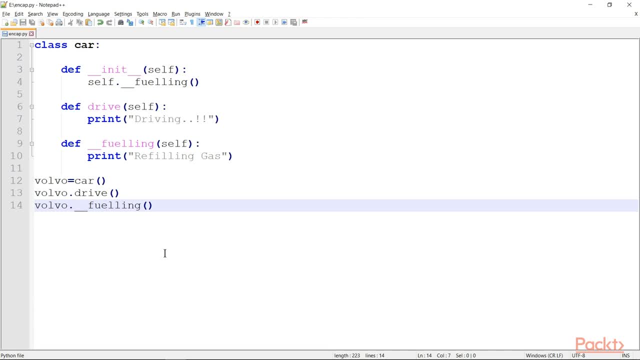 in which with an object declaration you have done, volvo equals to car. similarly, when you are calling a method, a method through an object which is specie locally, as a private method, you need to declare object name that is volvo, dot, singe, underscore car and then it will go with private methods name that is private. 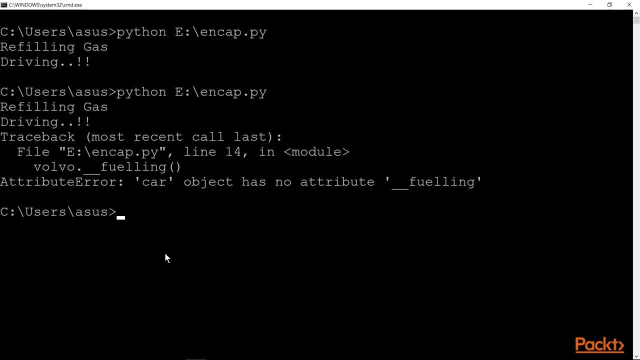 one, Okay, small as to that is double underscore fueling. let's save this program and rerun this program quickly. now that you can see is refilling the glass output as a print function is giving printed by in a declaration. second print command is: 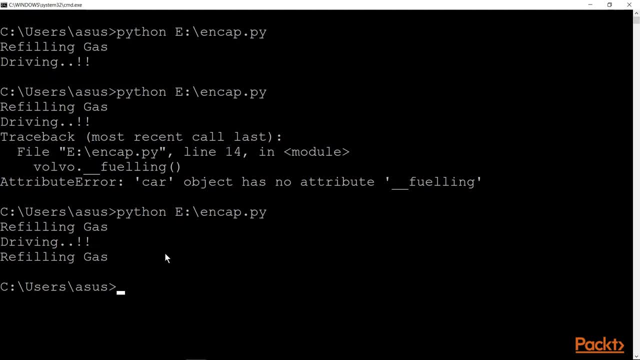 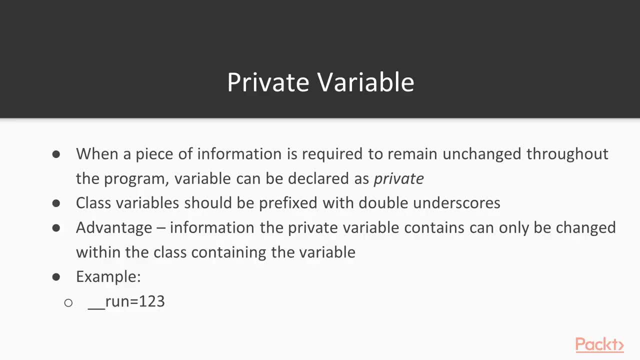 given by the method drive. and third, which we have called it through a private declaration, private method, which is through an object. similarly, we have private variables. when you want a crucial piece of information to remain unchanged throughout the running of program, you can define the variable holding set data as private, also by prefixing the variable name with double. 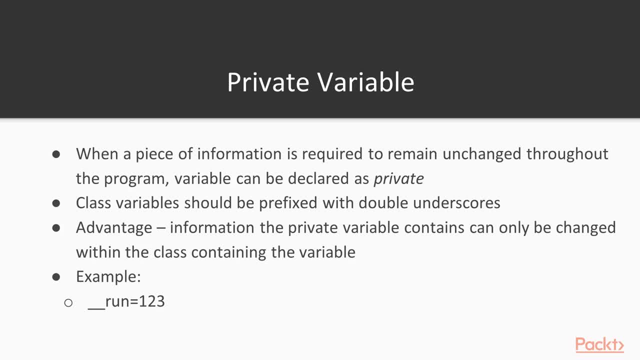 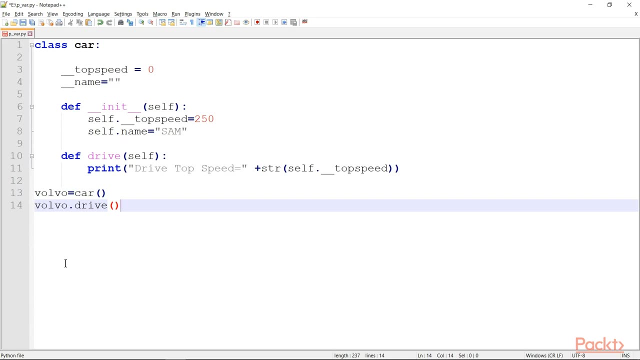 underscore. the advantage of assigning a variable as private is that the information the variable contains can only be changed within the class containing the variable and not outside. to summarize all of this, let's take a simple code. I have already written the code with the class name, car under which. 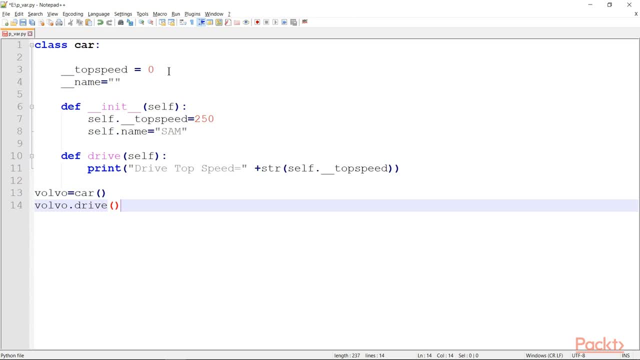 I have declared two variable names, with double underscore top speed, which is assigned as 0, and double underscore name, which is assigned as blank. then we have two methods. one is in it method and second is a drive method which holds a print command in it method. I have given a self declaration to the both the private. 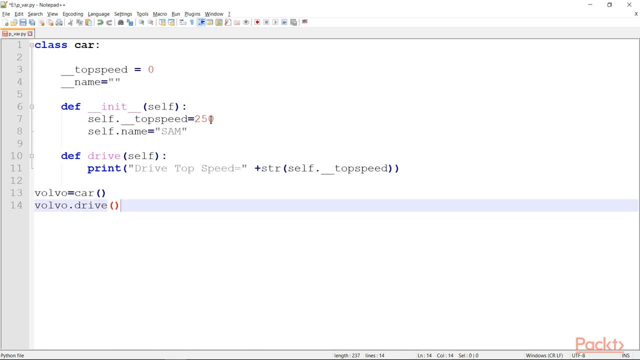 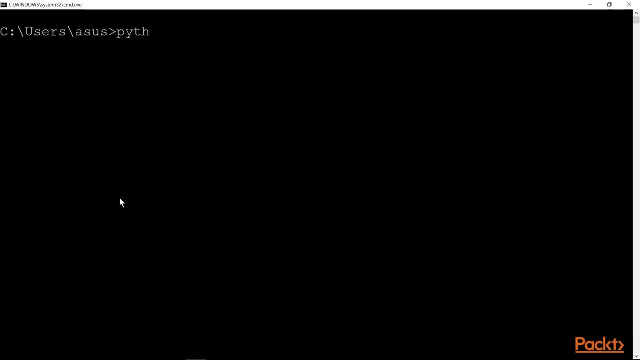 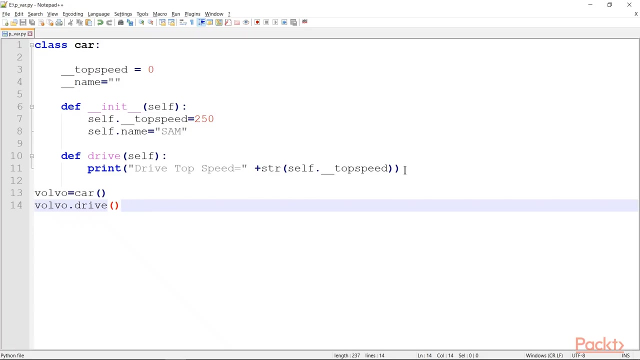 variable with the value of 250 for top speed and name with Sam. so let's try and run this code quickly from a command line. you now that you can see as an output you're getting a drive top speed as 250, which is defined in the code of init method. let's make a quick change to have 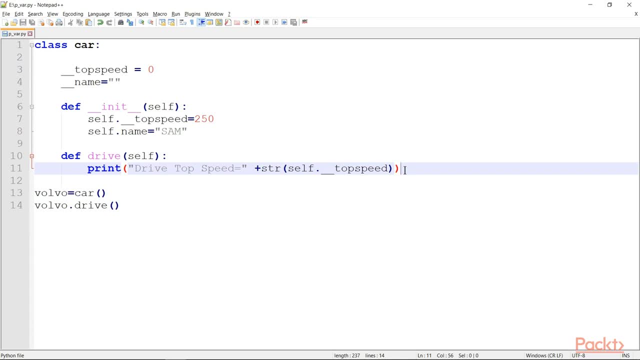 an access for private variable. with a change, you're writing an additional method that is deaf. set top speed with a self and a speed declaration as parenthesis. So we are setting: we are setting a variable name as top speed, which is connected to speed, as self declaration. 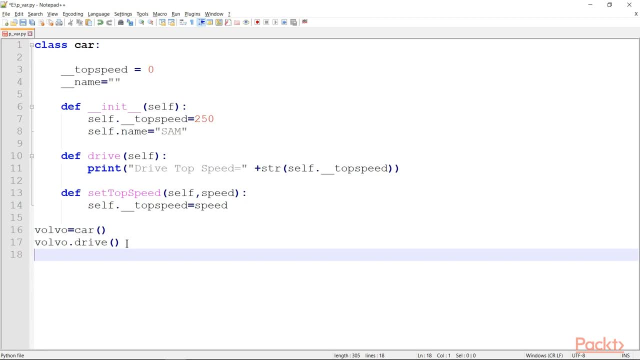 Now that we can push a value- parenthesis- directly through object, we can call set top speed with a value attribute that can be pushed directly through an object to have a value updated on our screen. we will also call the attribute drive, that is, the method through an object. 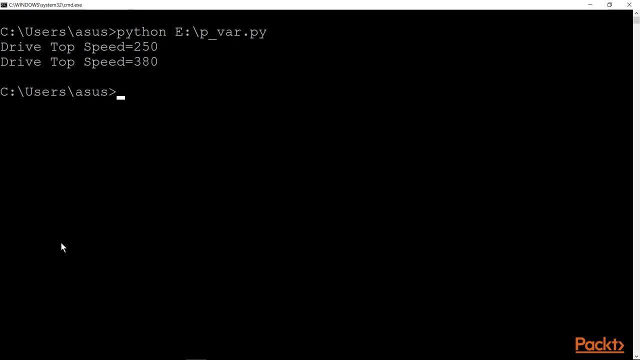 Let's save this program and run this program in the command line Now that you can see, the first drive recalls to the set value in init, that is, 250.. Then a set top speed gives you an access and through object we can push the parenthesis.